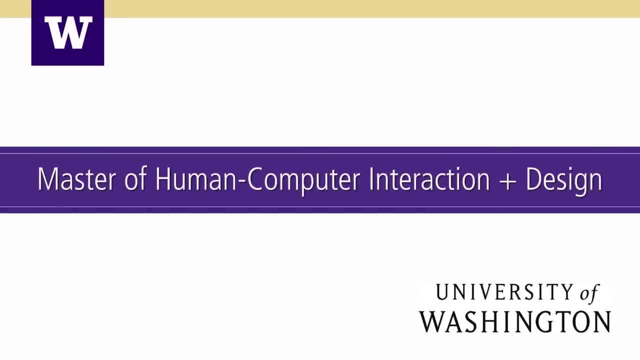 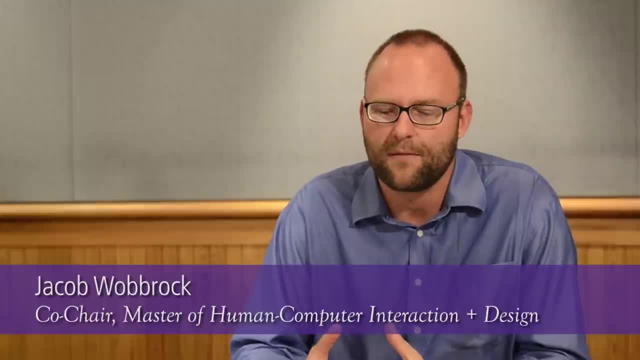 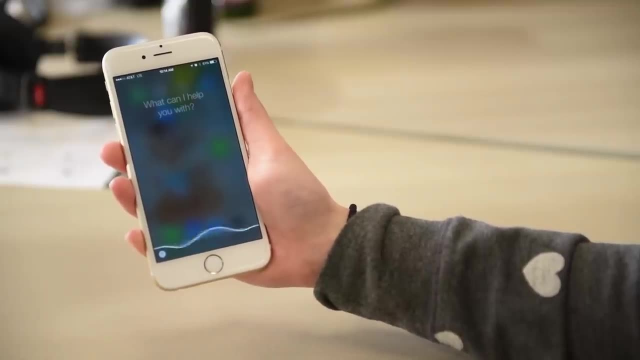 Our human-computer interaction and design program, I think, is ideally positioned to make a big impact in the world right now because, as more and more products and services come out that are consumer facing and really involve the marriage between technology and people, we have to get that design. 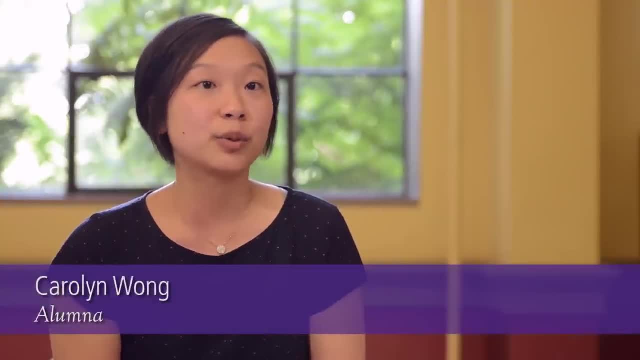 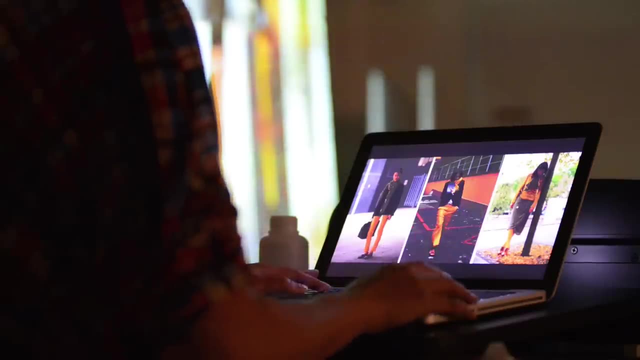 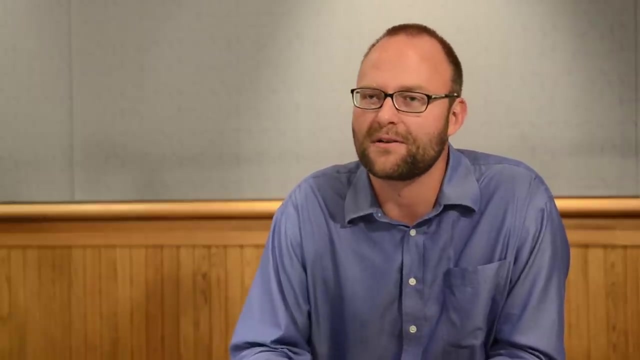 right. I think overall the industry is maturing. so before in technology if something worked it was magical, like it's cool that it works, but now, like people just have higher expectations of what will delight them, what will surprise them. The MHCID program is a cross-departmental, interdisciplinary 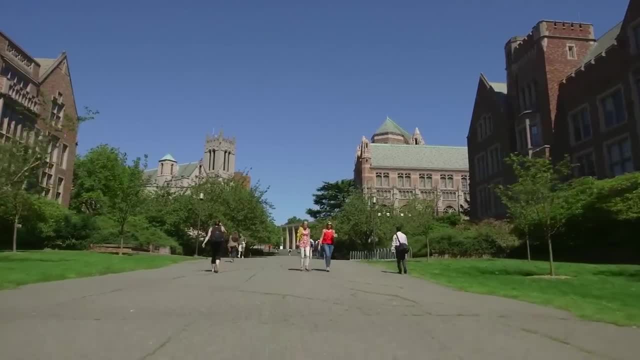 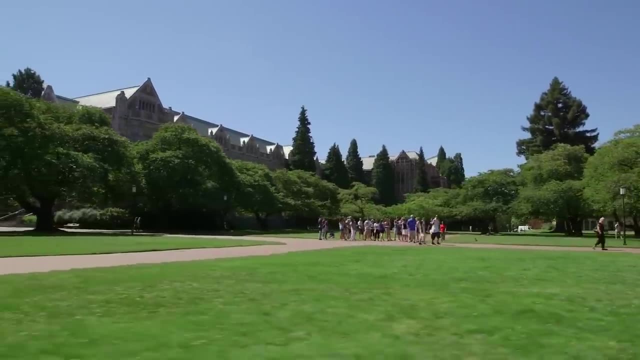 program that is not owned by any one department, and the four departments that contribute faculty time and resources to the program are the Information School, where I come from, the Department of Computer Science and Engineering, the Department of Human-Centered Design and Engineering and the Department of Computer Science and Engineering. 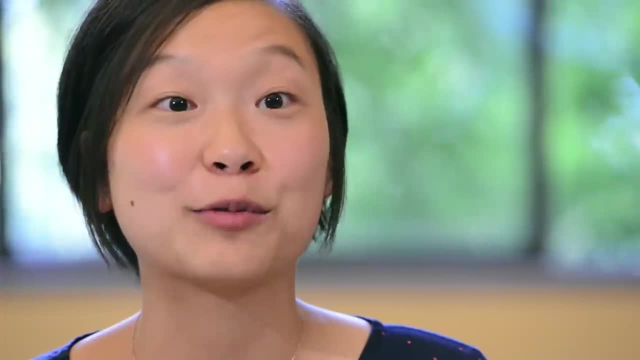 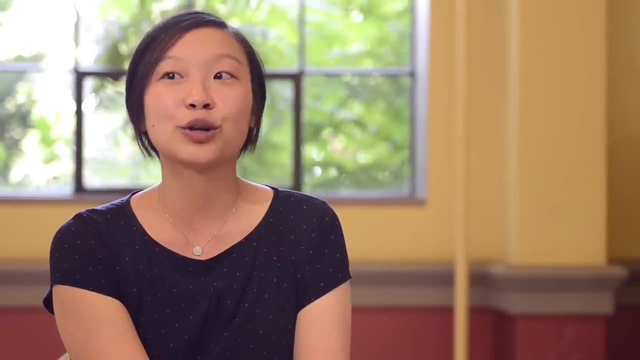 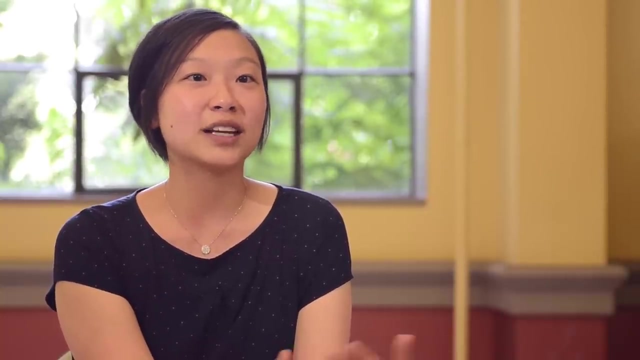 The Division of Design within the School of Art. Coming in, I was totally surprised at the caliber of who was teaching our program. so there's at least two or three professors I know in the past two years that were under in the list of like 30 most innovative under 35. They're like the people who 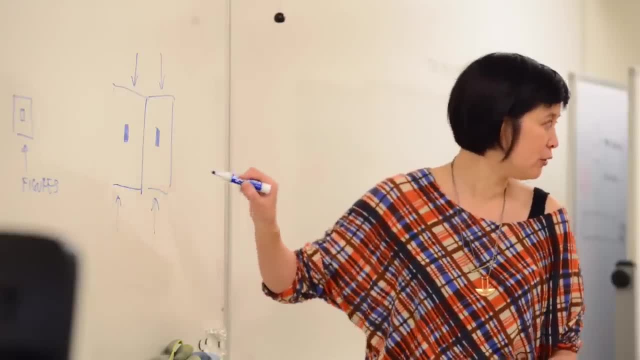 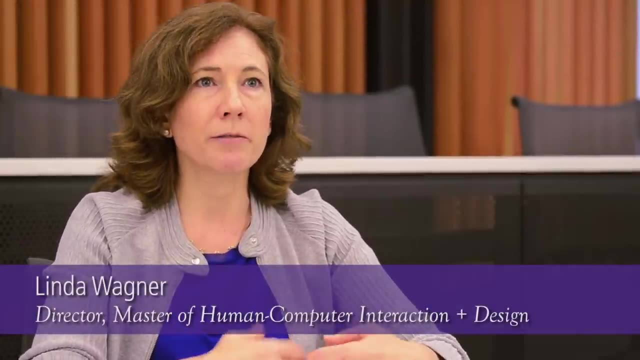 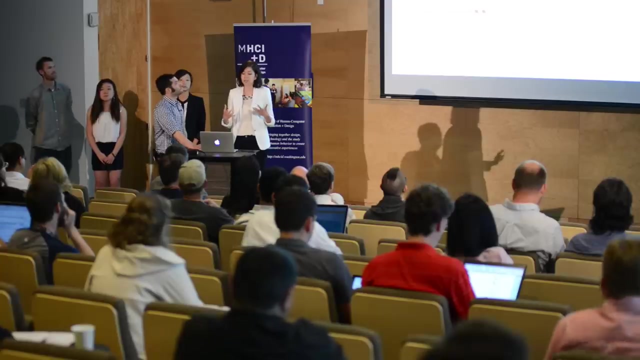 wrote the book on input, on ubiquitous computing, on persuasive design. One of the nice things about this program is that it, I think, is more reflective of the workplace, in the sense that we recruit people from a variety of different backgrounds and perspectives and we bring them together. 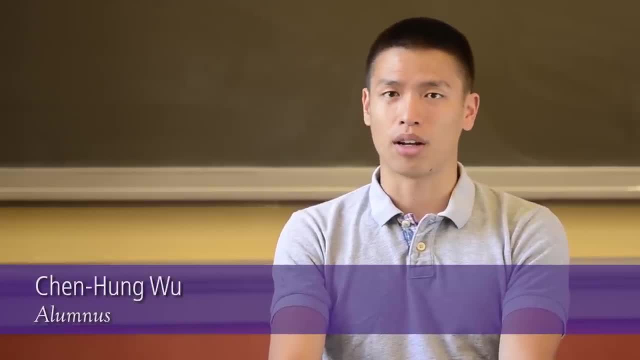 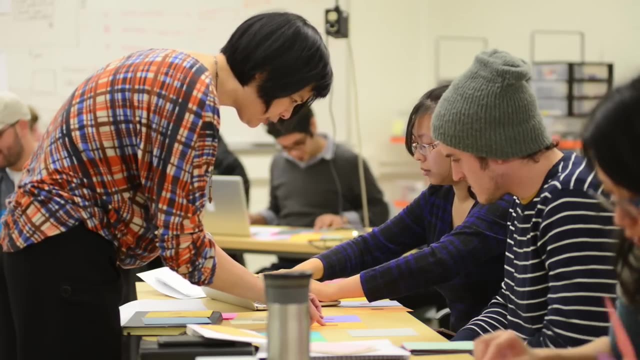 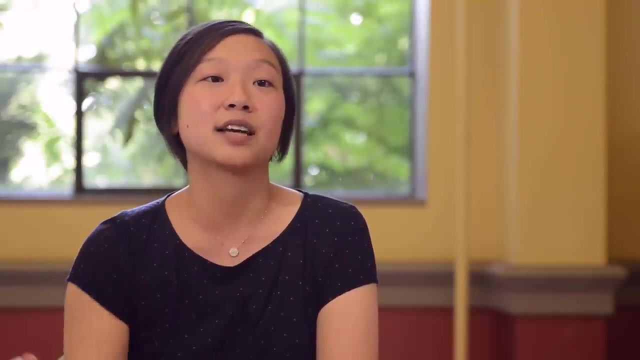 It's a one-year program, project-based. It's basically centered with a studio class and this studio class actually emphasizes on lots of hands-on work. Our curriculum is focused on three specific sections. so one: research, so learning about the psychology. and how about people? how do you really understand and get at? 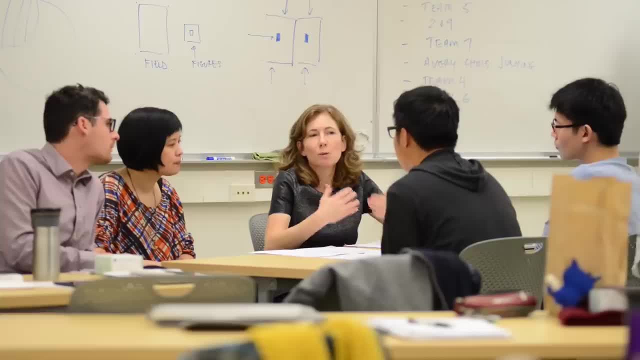 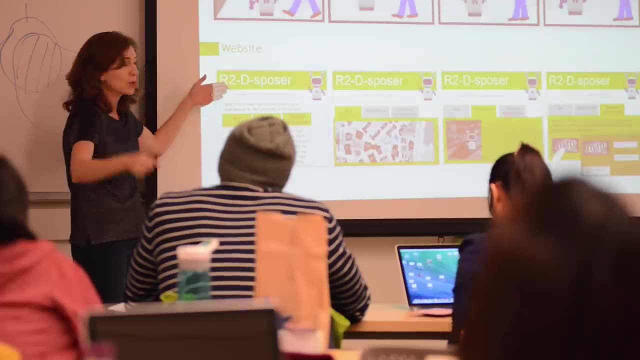 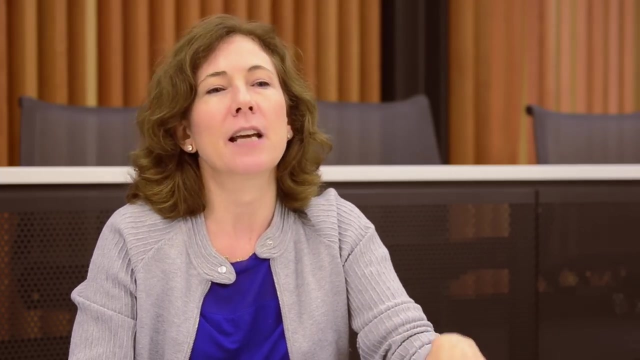 what people want and need, what their pain points are, and then from that how do you ideate a create or create a solution to meet those needs, and then prototyping and technology learning how to actually execute on those types of ideas. The Capstone Project is an opportunity to take all.